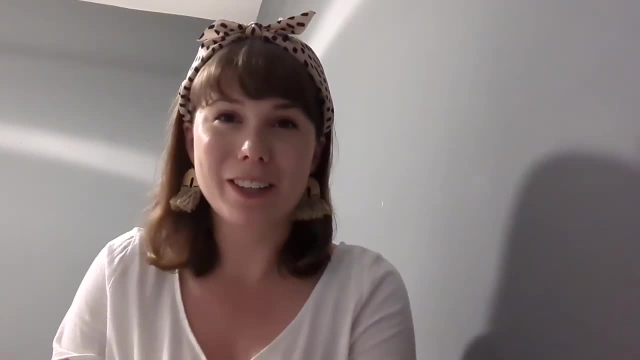 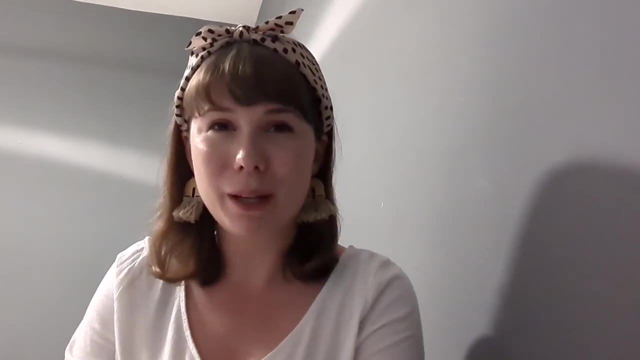 Being an international student from the States and London has been pretty great so far, to be honest. It's been really fun to explore all the little culture differences, Obviously like there's a lot of similarity but there's a lot of differences too, which it's just really exciting when you find. 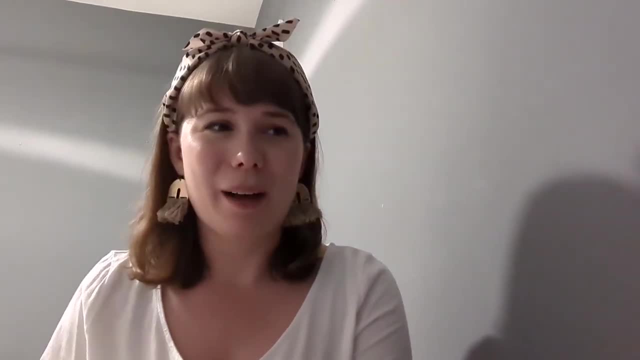 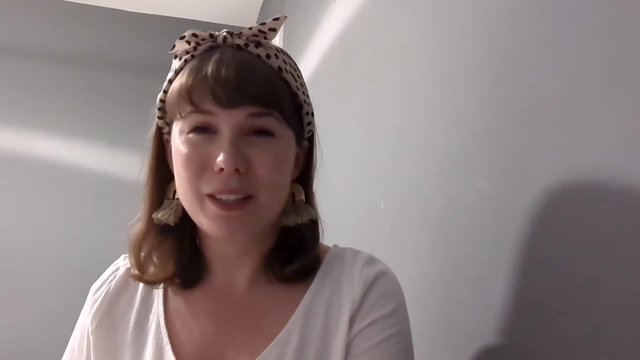 those and you get to learn new things. As far as school goes, the school is pretty similar. The language is obviously the same, which is really nice. Some of the differences are the way that grades are given here and also the amount of assignments you're expected to complete. So back. 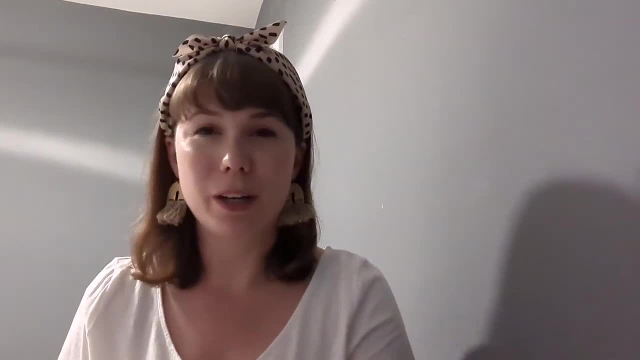 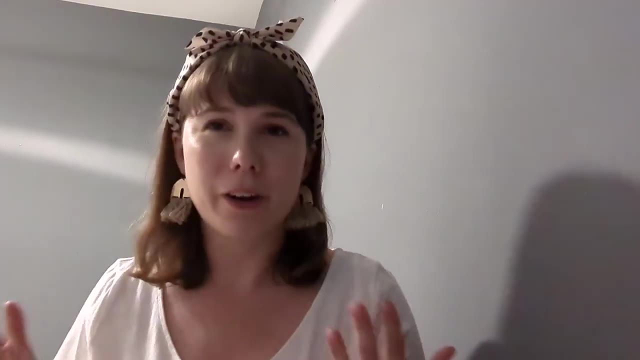 home in the States, we would be given kind of constant assignments throughout a course, but here, a lot of times, you'll have one project and one exam, or maybe just one or the other. that makes up your entire grade, so that's a little bit different. The program, though, is also shorter and more. 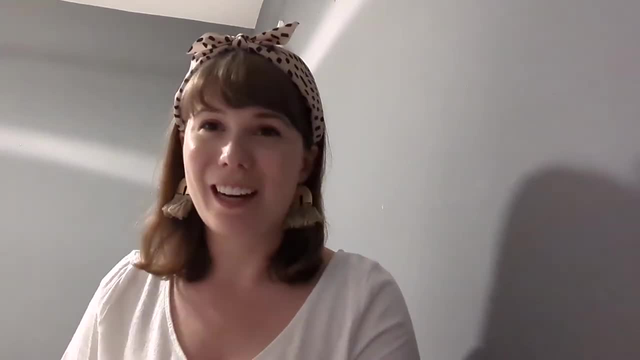 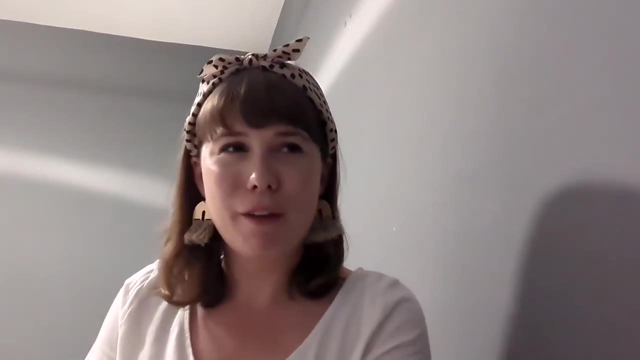 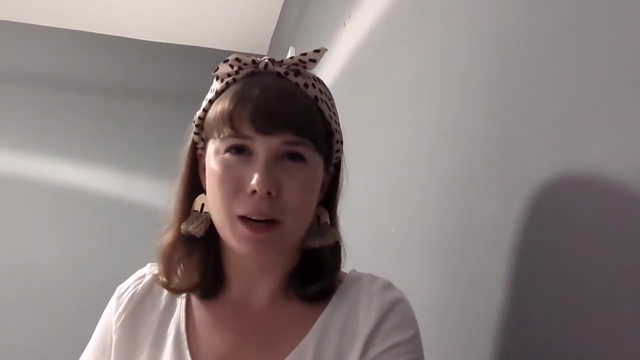 affordable than similar programs back in the States, so that's really nice. But yeah, overall it's been a really cool experience. I think my favorite module was actually the very first one I had, Interaction Design. It covered all the basics of the user-centered design process from start to finish, and the coursework was a project. 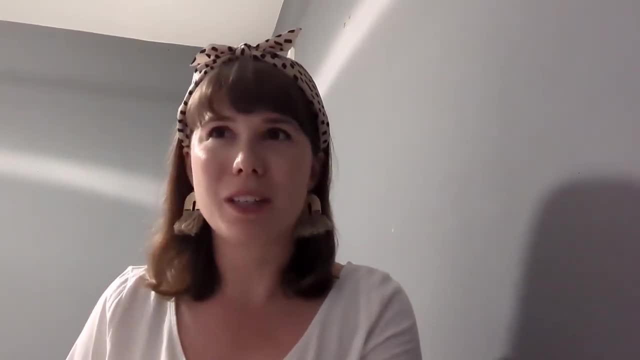 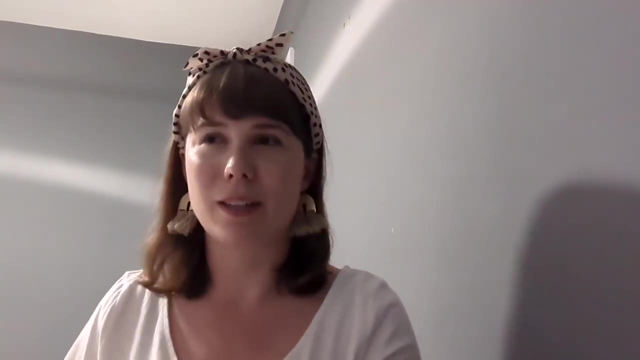 where we went through the entire process. So that was really cool to just see the entire thing kind of play out and be a part of that and just really learn what it would be like to be both a UX researcher and a UX designer at a company in a real job. So I think that was really useful. 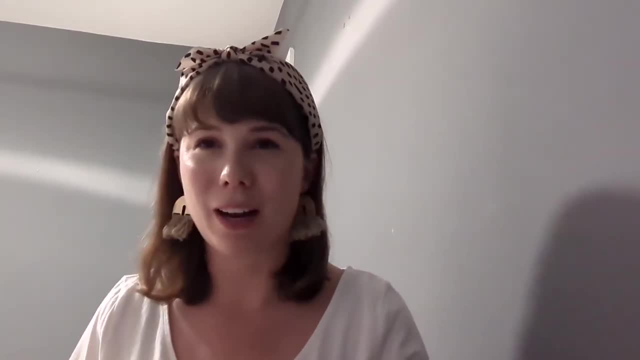 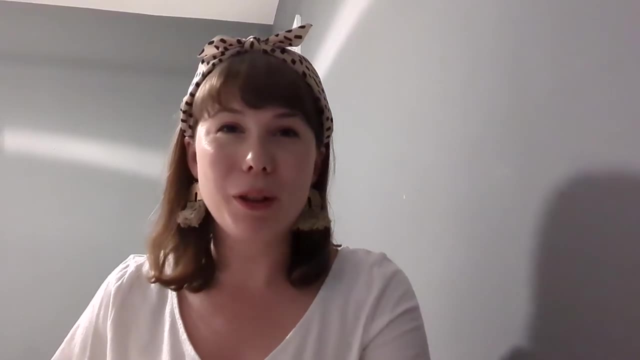 for me to get a sense of do I really like this and what will it be like when I graduate? And so, yeah, I'm really glad I took that one. Throughout the program we've had a lot of opportunities to create realistic work that we could put in a 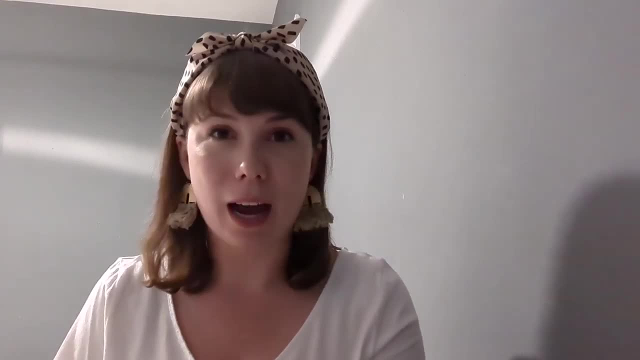 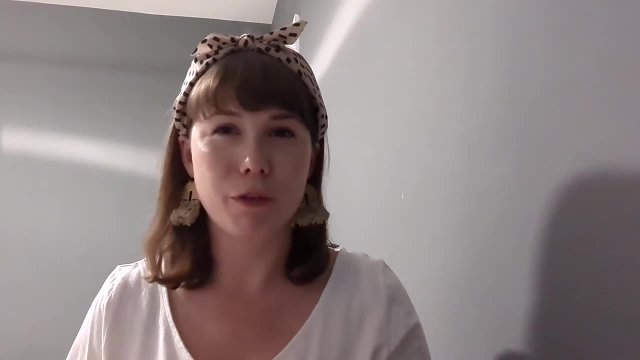 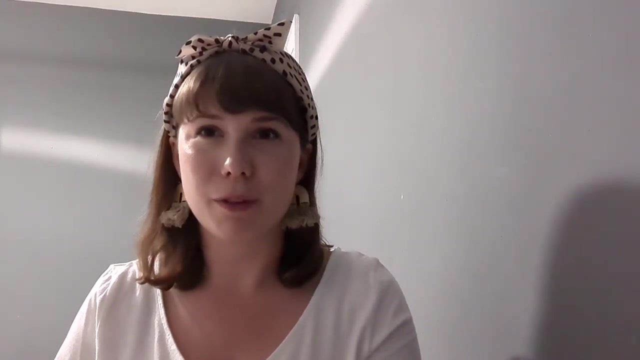 portfolio, whether that just be tutorials we've done in class or final coursework that we've worked on throughout the whole term. So I think being able to create that tangible work to show future employers really helped set me up for success. I also think that Citi has given me a lot of those you know: technical skills and designerly. 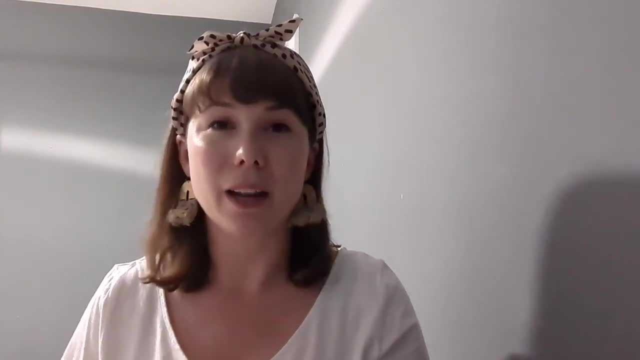 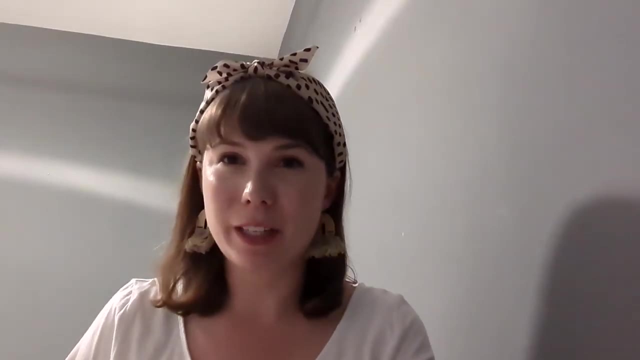 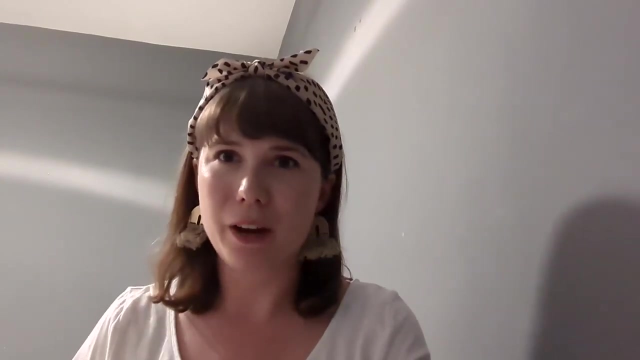 skills that I would need to you know understand how to excel in the UX field. I'm really interested in voice user interfaces, which, you know, isn't necessarily a super new concept but it's really expanded in the past few years with, you know, Amazon, Alexa and Google Home.